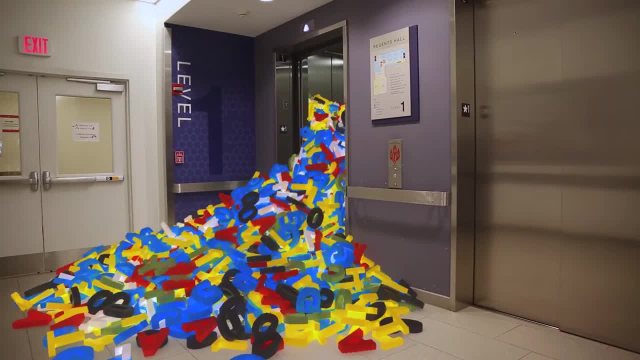 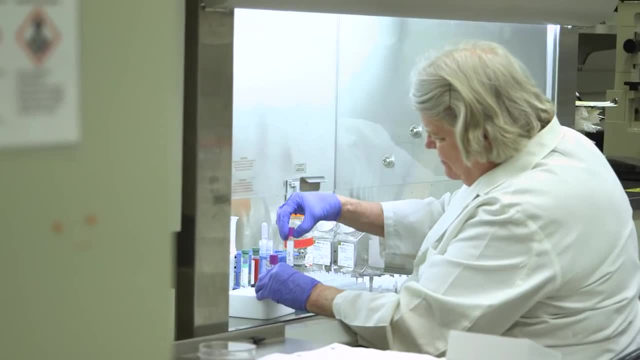 workforce of data managers and data scientists to analyze and manage this data, and even find a way to provide adequate storage for the mind-boggling amount of data being generated by scientists, researchers, governments and private companies. The field of genomics is the fastest. 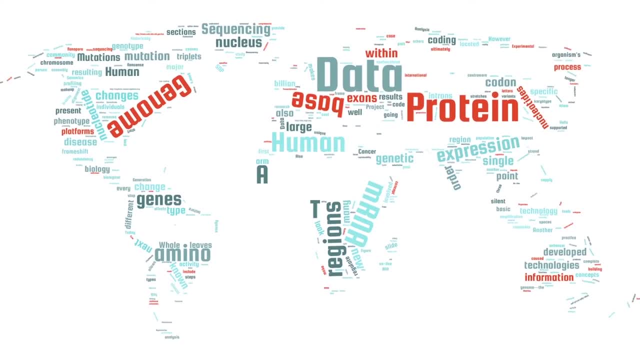 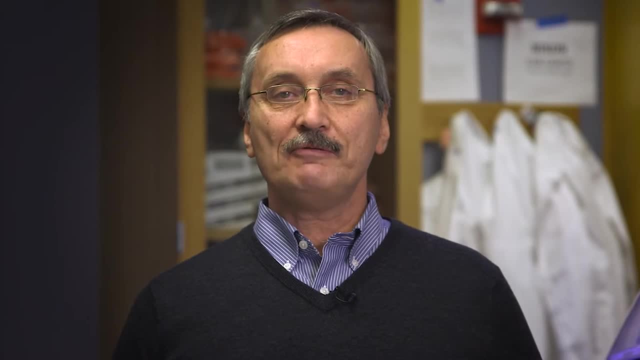 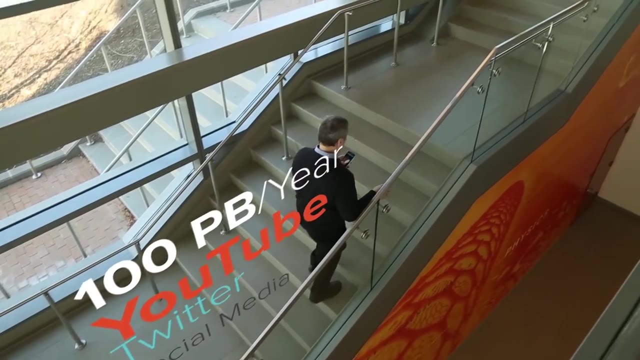 growing data generator in the world today, with the quantity of genetic data being produced on a daily basis doubling every seven months at the current rate. By 2025, the amount of data generated by genome scientists will surpass that of YouTube, Twitter and the current reigning data kings in. 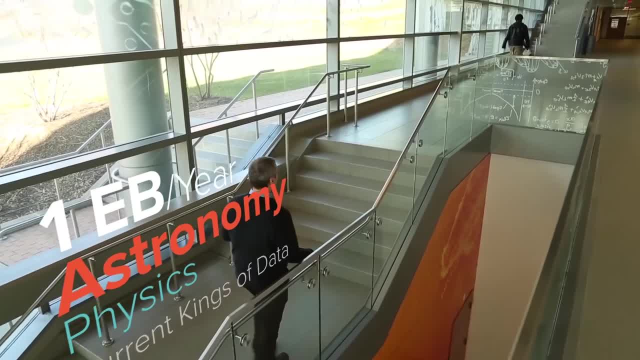 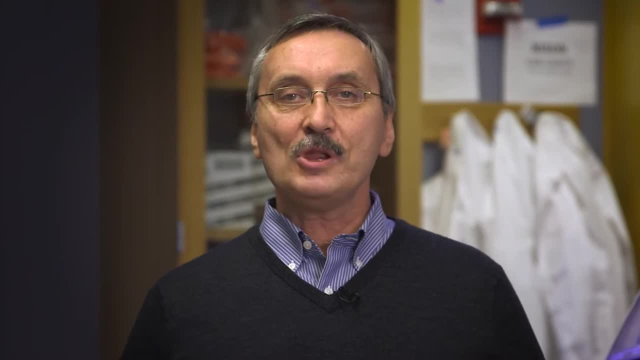 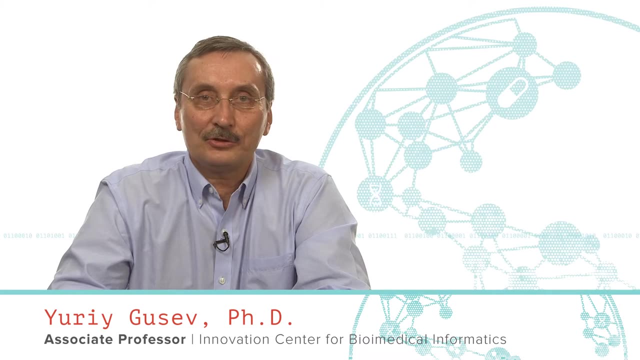 science. In the next 10 years, researchers will be producing somewhere between 2 and 40 exabytes of data every year. In order for us to take full advantage of the biomedical big data that we are accumulating, we need to understand it and learn how to analyze it. For this reason, we have created a free online 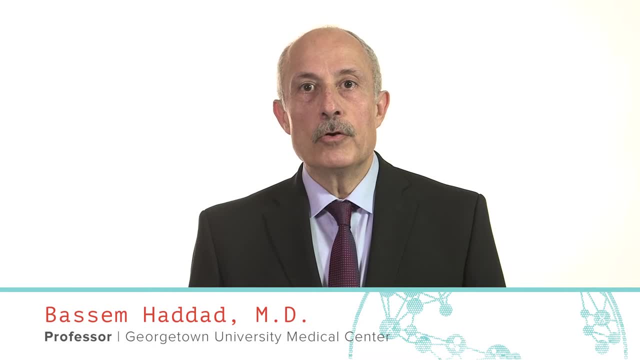 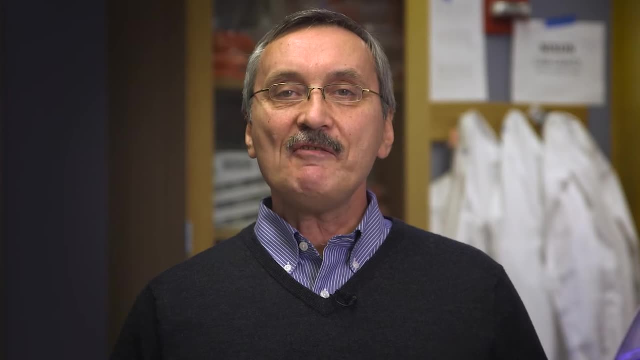 course that will provide you with a broad understanding of the biomedical big data and hands-on training in the most recent databases and analysis tools. This course covers seven major types of biomechanics. The first is the biomechanics of the human brain. The second is the biomechanics 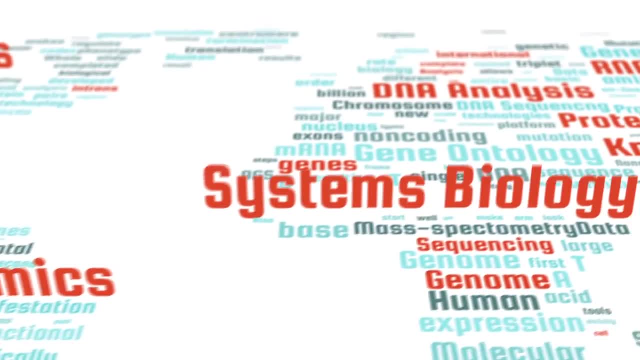 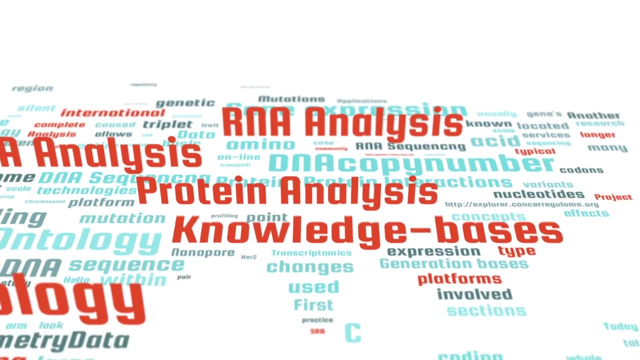 of the human brain. The third is the biomechanics of the human brain. The fourth is the biomechanics of biological data in genomics, transcriptomics, proteomics and system biology, including data types generated from DNA analysis, RNA analysis and protein analysis, as well as biological knowledge. 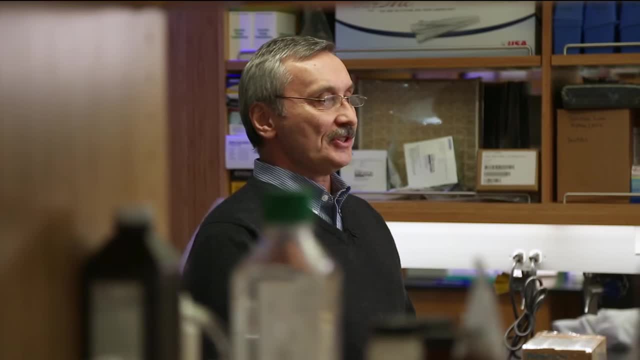 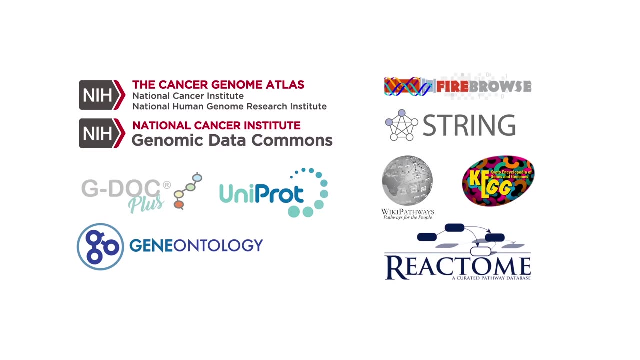 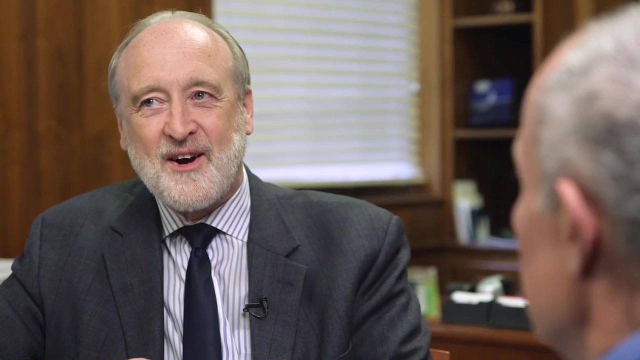 bases, pathways and networks, Along with lectures and software demonstrations of the most well-known open data resources, such as TCGA, GDC, GDOC, UniProt, Go and many others. you will listen to leaders in the field discussing important applications of biomedical big data in 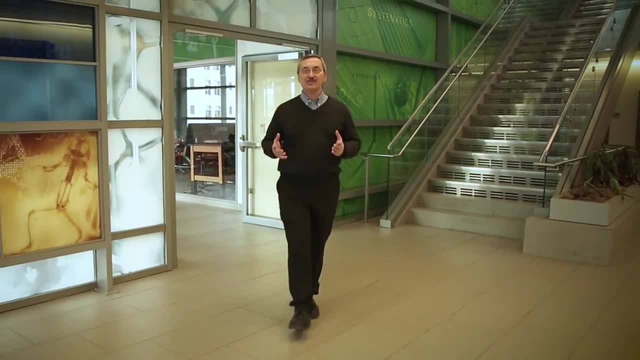 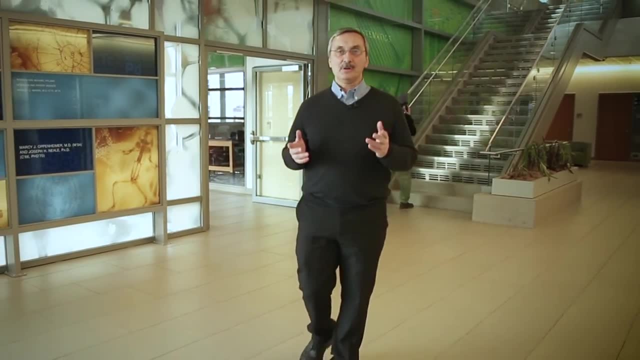 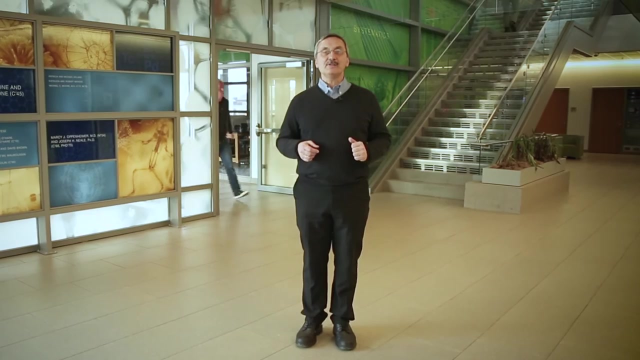 biomedical research. As this field is continuously changing before our eyes, we will continue to update our course modules as new information and new tools become available. This course is intended as a living resource for a new generation of biologists and clinicians seeking to learn how to leverage open and freely accessible online resources. 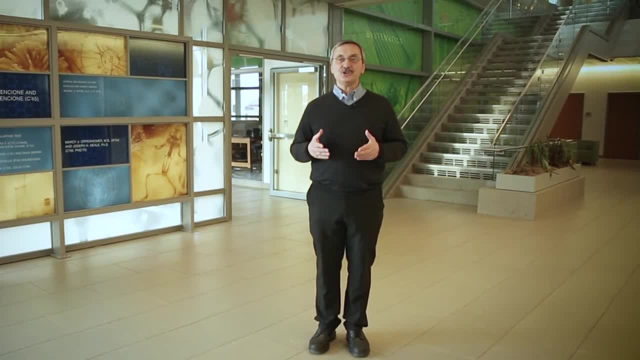 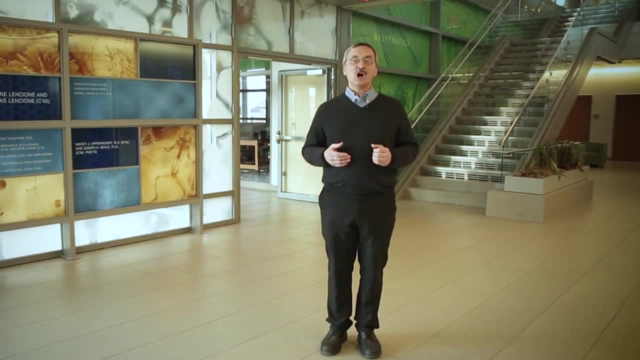 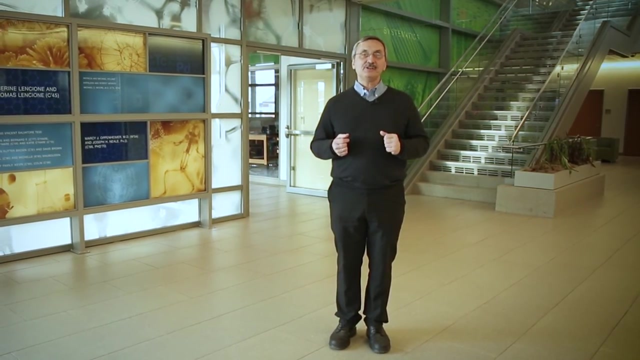 and tools for clinical decision making, translational research and to make important new discoveries, as well as for the general public interested in learning more about how biomedical big data is transforming the field of medical research. Our goal is to demystify this field for you.